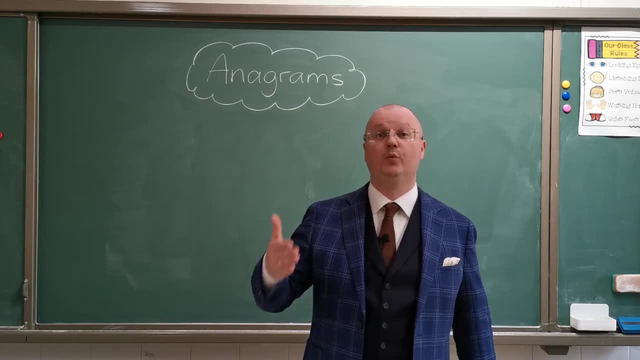 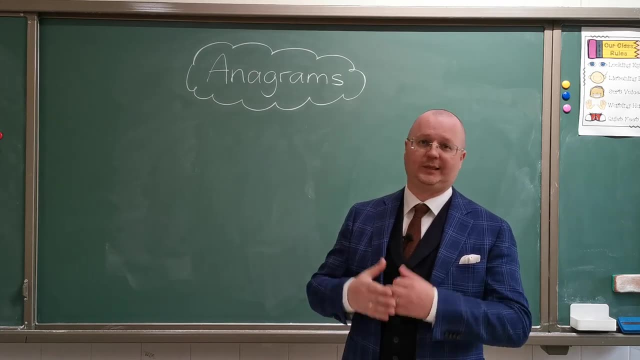 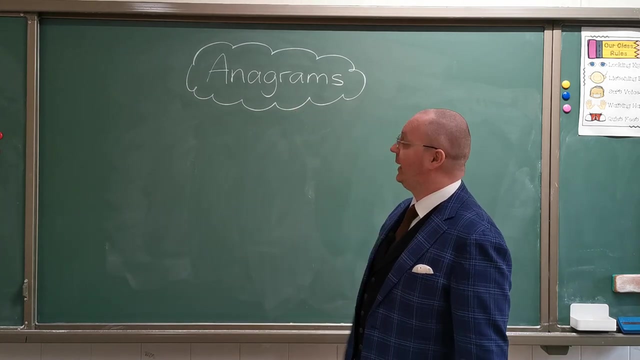 So we do a warm-up activity to set the mood, to tune them in to the learning mode. That's why we say that your warm-up activity doesn't have to be the same as the topic of your class. This activity is intended for grade. 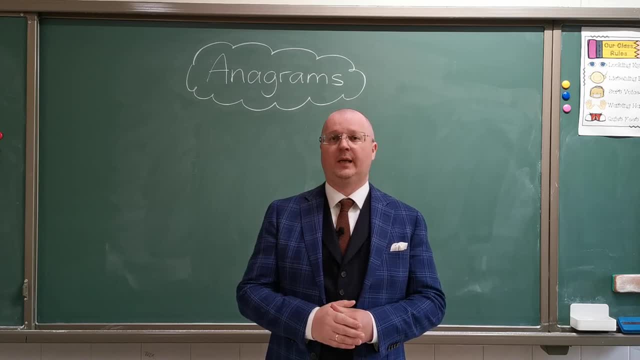 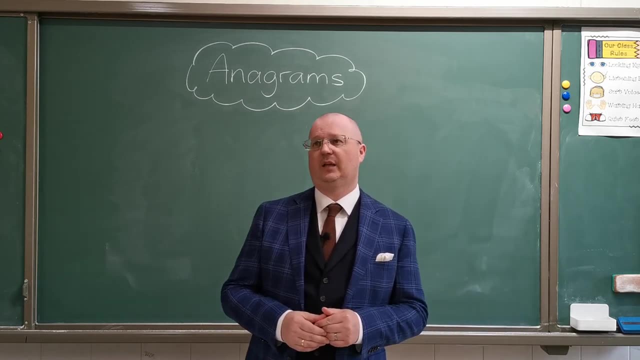 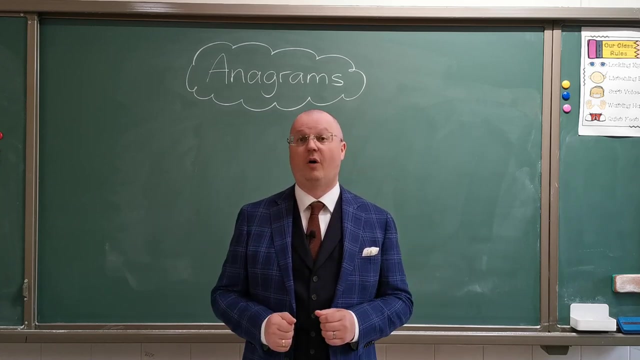 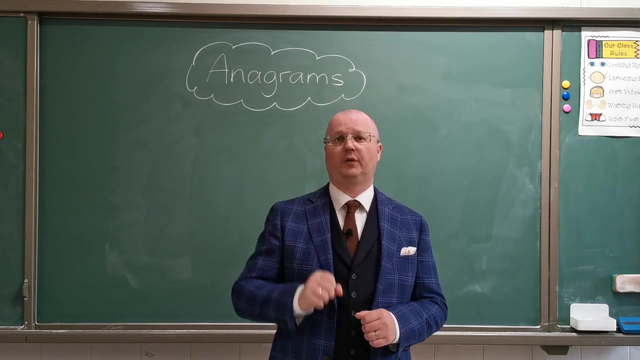 maybe four, five, six and above, Because it's a vocabulary building activity And also I think it's a good one If you want to introduce the topic of your class. If the topic of your class is a long word, You know, like if we go through the structure of the lesson. So the very first thing we do 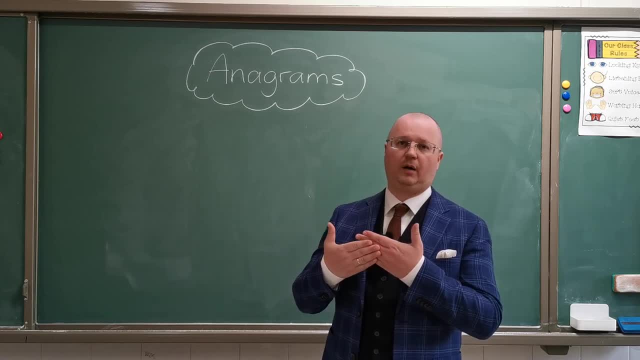 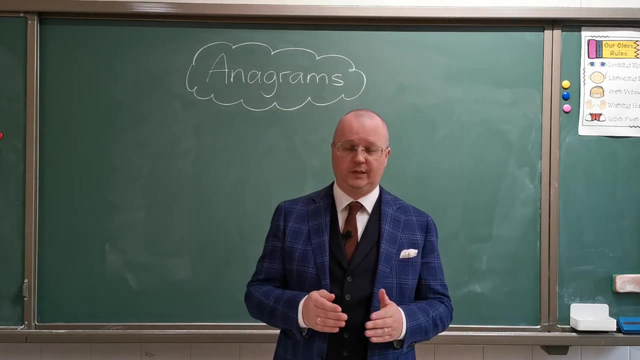 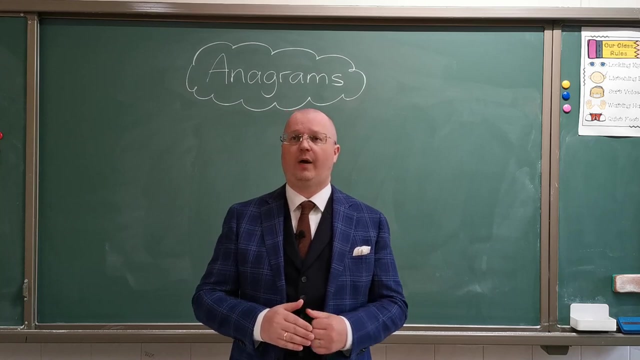 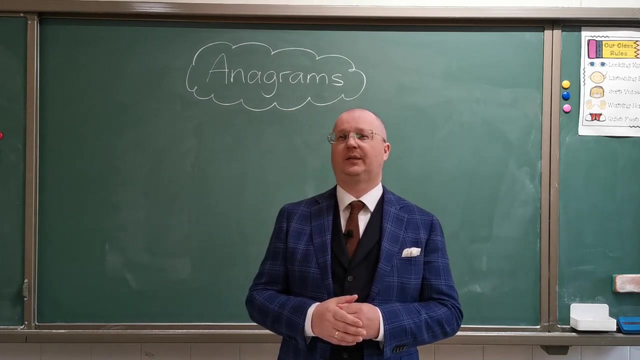 we greet the class Number two would be your routine, Like in my case. I always split my students into two teams. We go through the rules And then I start the class. class also after you do the warm-up, then you do a review and then there is like sometimes 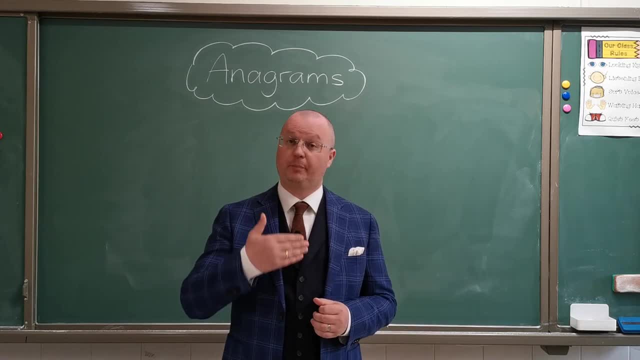 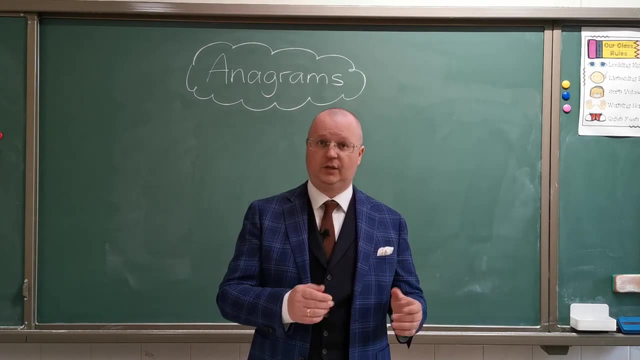 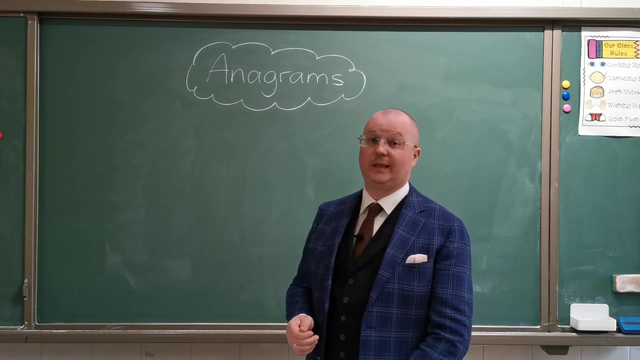 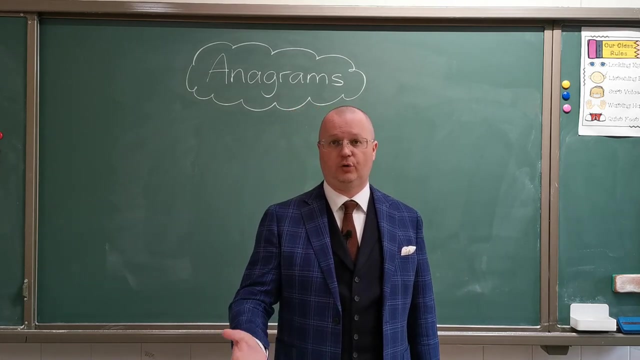 sometimes teachers do what they call pre-task or pre-teaching activity. this is where you introduce your topic and you try to connect the topic to what students already know. so I think you can use it as a warm-up or you can use it as a pre-teaching activity where you introduce the 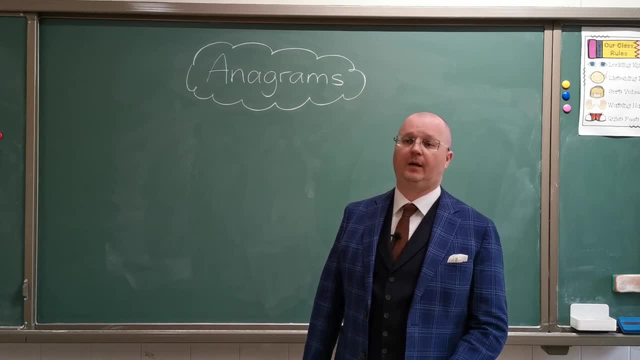 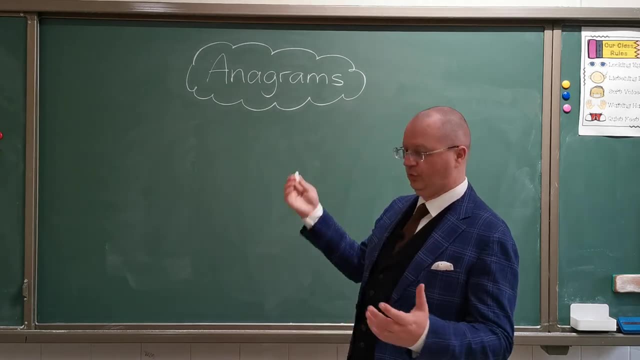 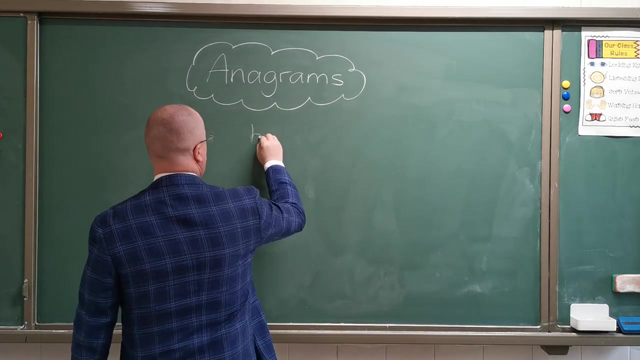 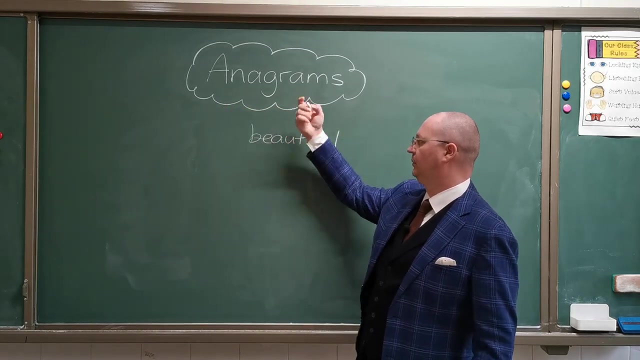 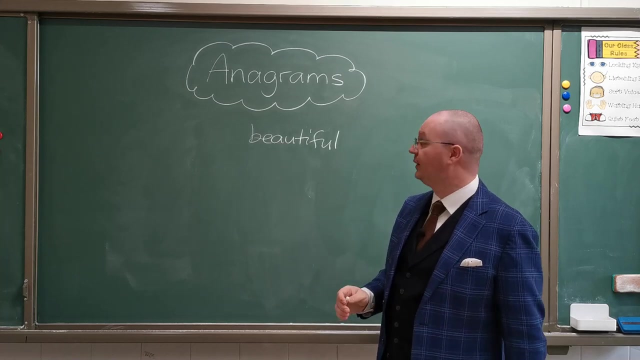 topic, provided that the, the word is long enough. so basically, in this activity you need to, like, you choose a word, any words, for example, I don't know, beautiful, yeah, oh, let me write it: beautiful, beautiful, and and then, well, the meaning of the word anagram: you use the letters of this word to make as many words. 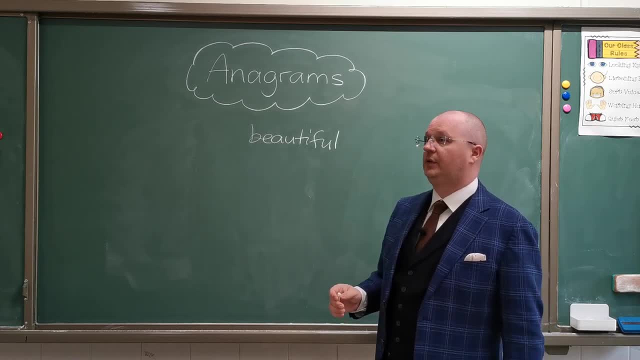 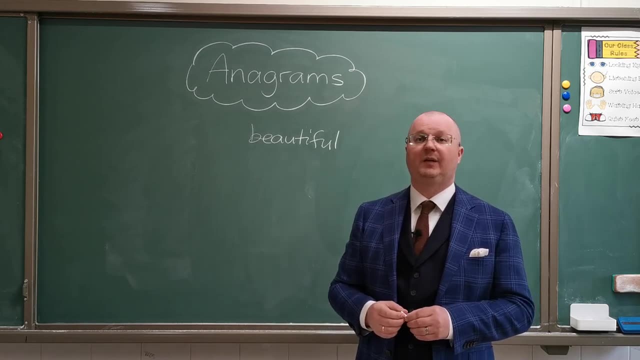 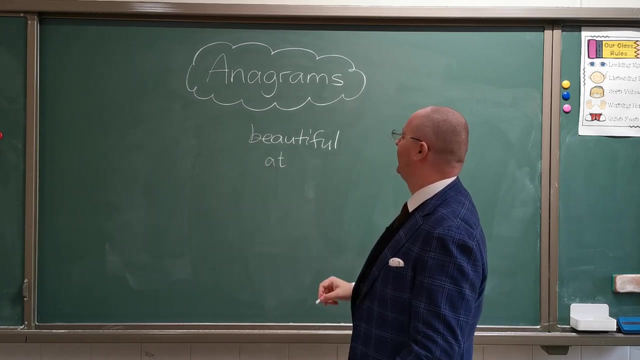 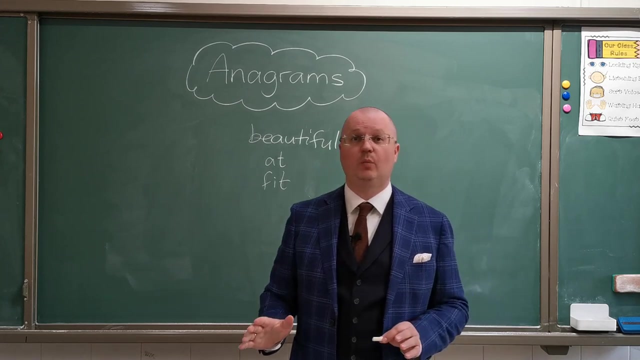 as possible, and you can do it this way. you can, for example, divide, you can invite a student from each team and give them one minute to make as many words as possible, for example at: at, that's a word, f-i-t fit, that's a word. so they have one minute to write as many words as possible. 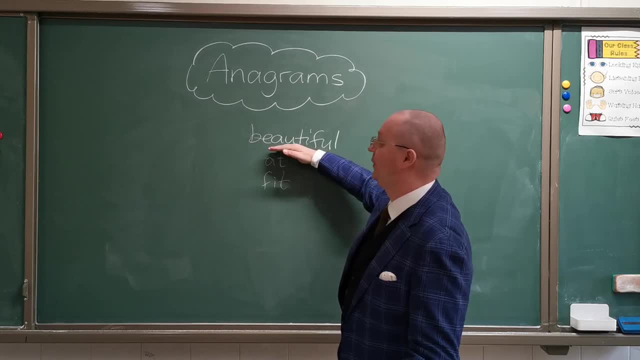 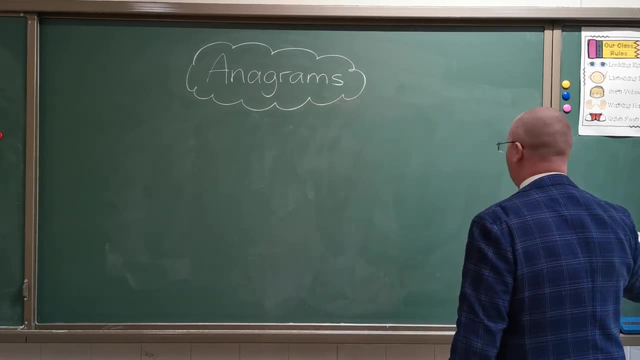 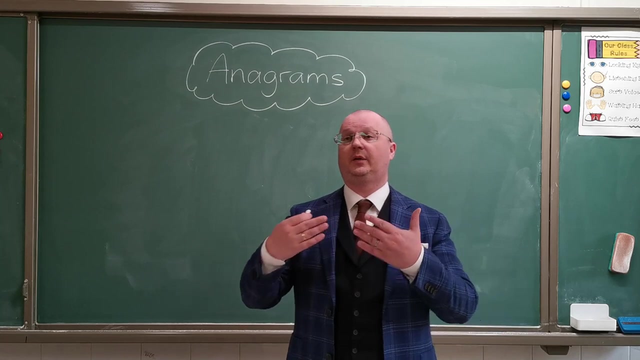 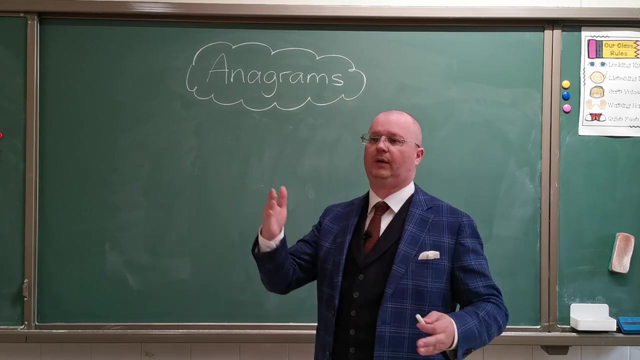 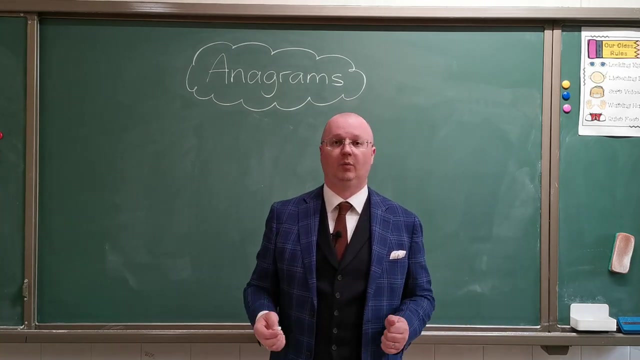 using the letters from this word. so actually I'm going to give it a go and let's see how many words I can come up with right. so, for example, let's say you're teaching Halloween, so you can write down Halloween. invite one boy, one girl, or like a student from each team. give them a minute and they would need to write as many words as 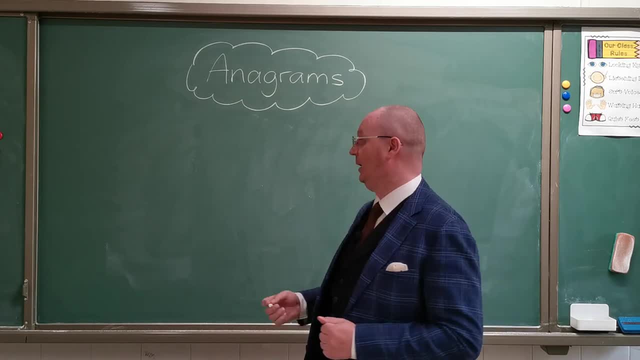 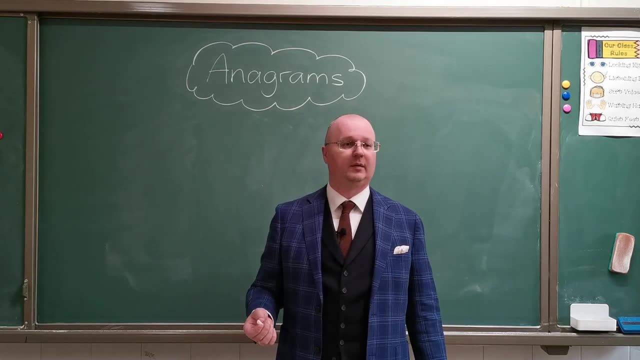 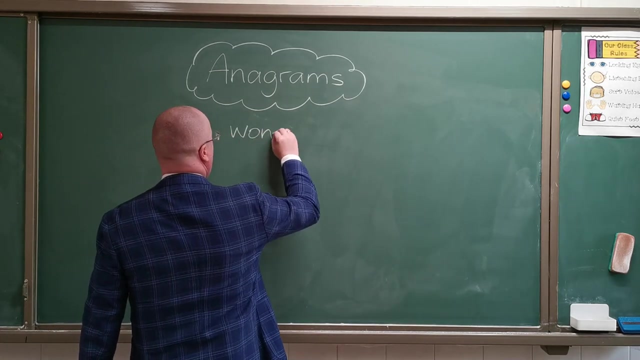 possible using the letters in the word Halloween. so let me demonstrate it and I'll choose, I'll pick, I'll pick, I'll pick. the word wonderful, for example. it's long enough, so you write the word wonderful here, yeah, and then you can write down the words that you want to write down. so let's say you're. 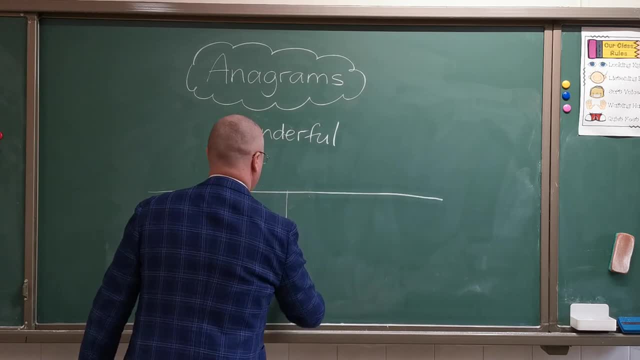 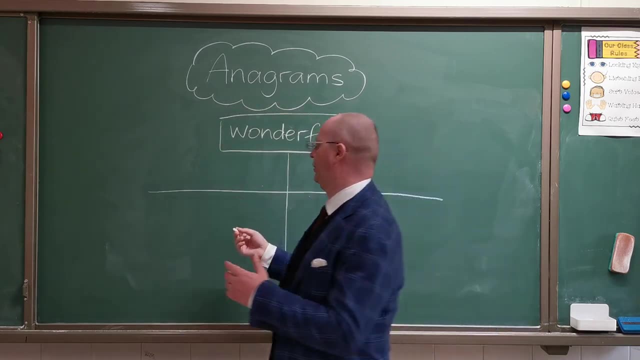 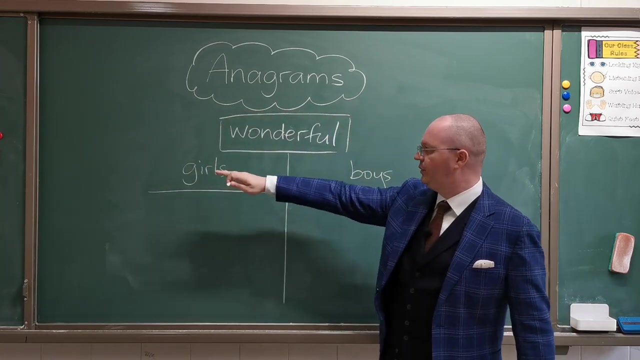 writing down the words that you want to write down and then so this would be your word, and then this the. this would be, for example, girls here and boys here. I am choosing to write girls and boys because this is what I do in my classes, but in your 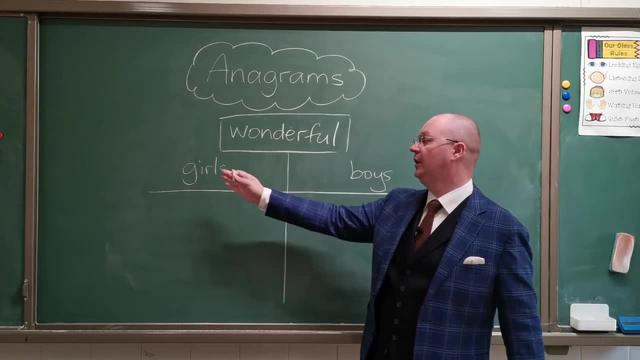 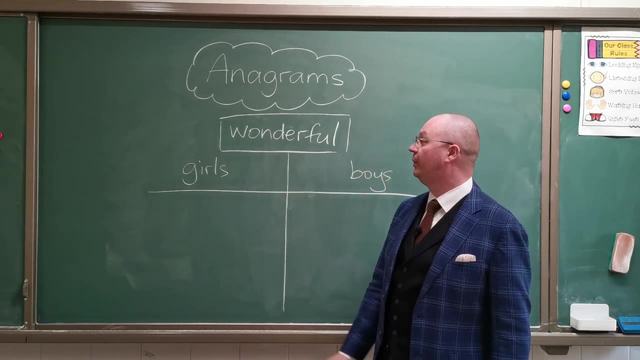 classes if you split them into two different teams. you can do it this way. all right, and let's see what we have here. so let's say you're teaching Halloween and you can write down a word. let's see how many words I can come up with using the letters from the word wonderful. so I have one. 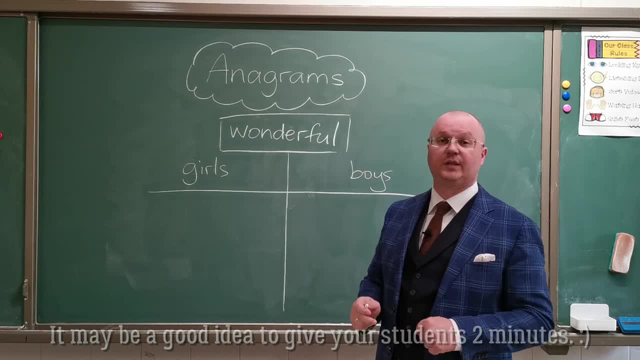 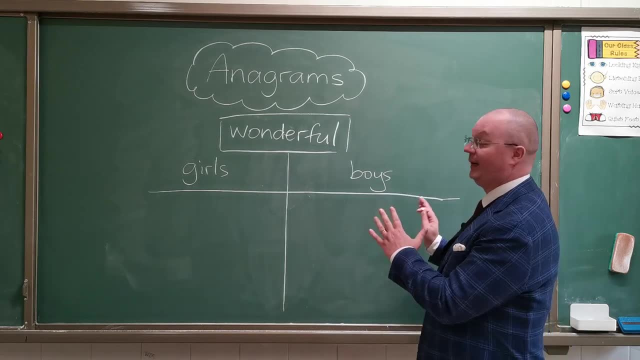 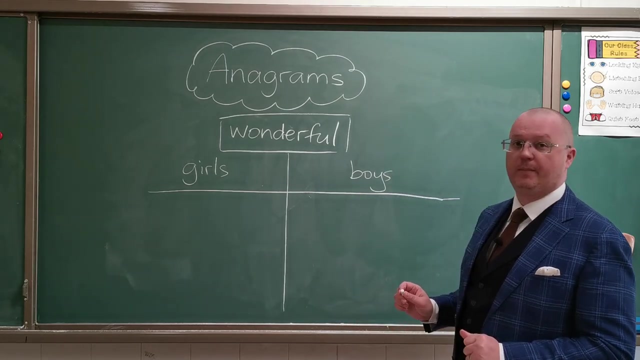 minute and in class, like the teacher, would set the timer. and also, if you like, you can invite not just one student, you can invite two students or three students so they can work together, you know. so let's just try, let's see how many words I can come up with in a minute: one, two, three go. 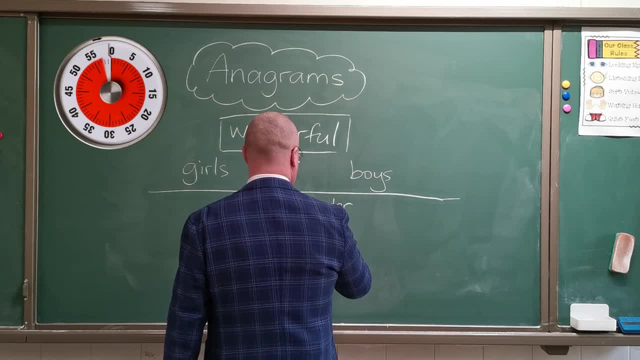 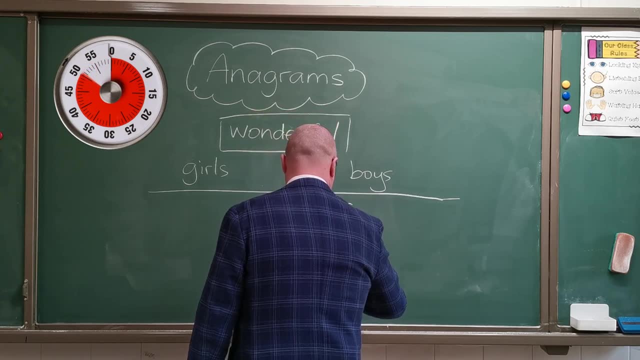 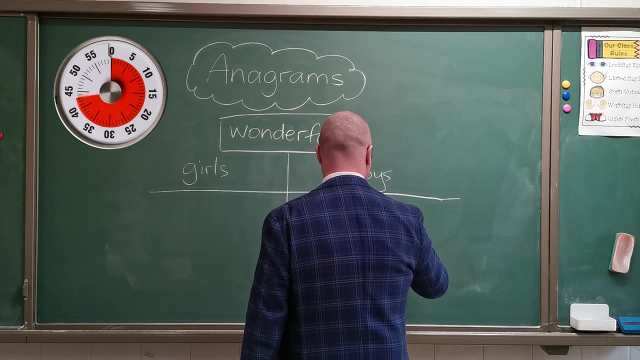 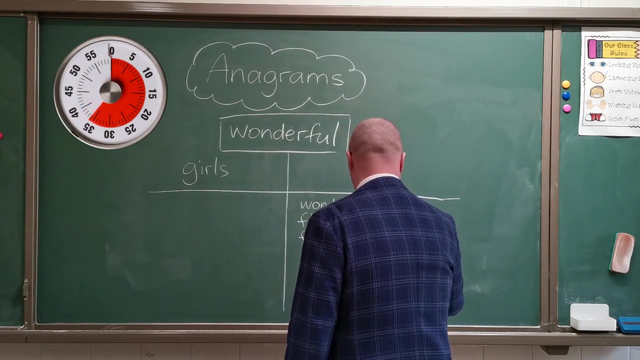 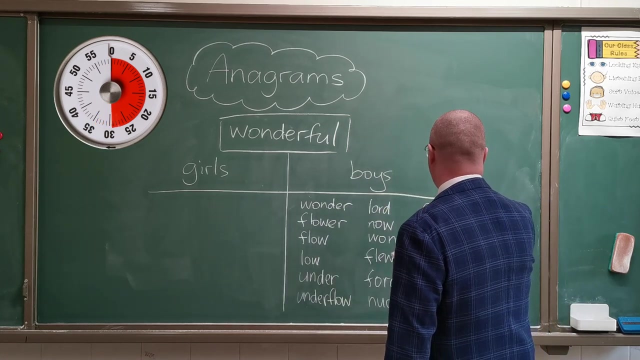 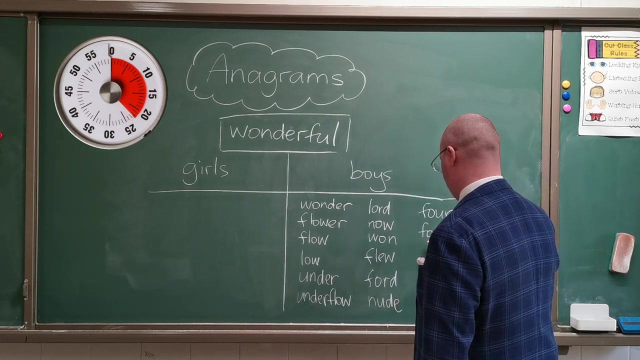 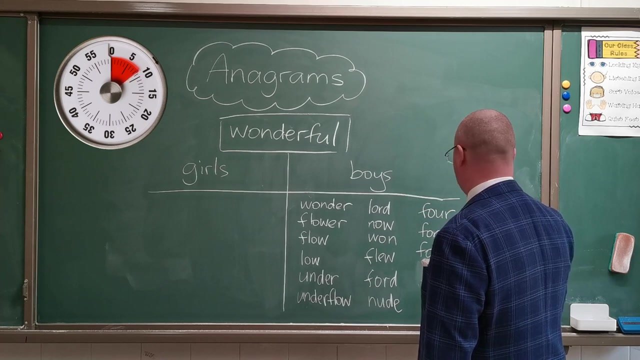 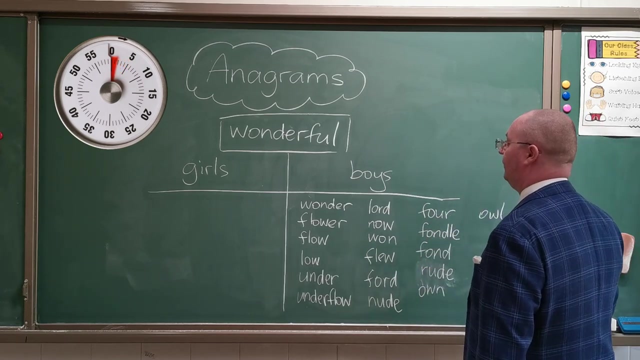 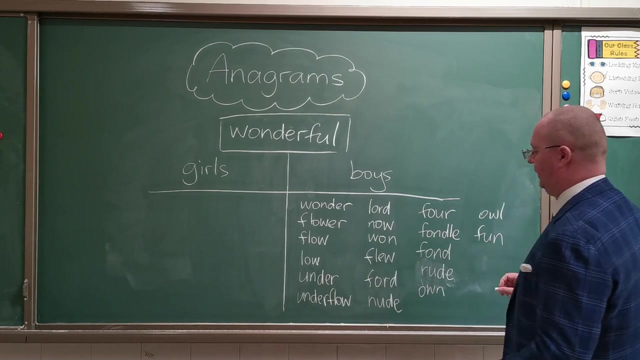 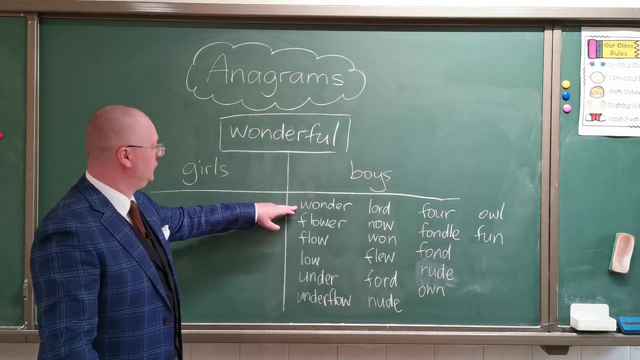 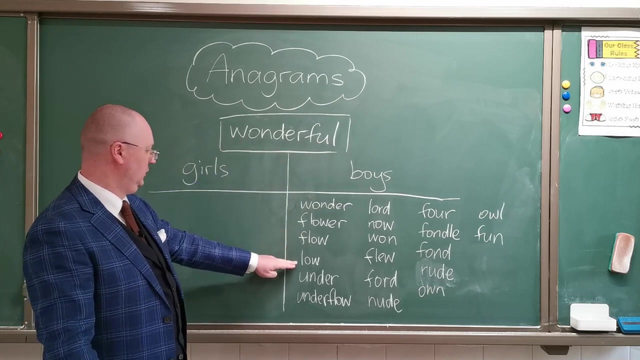 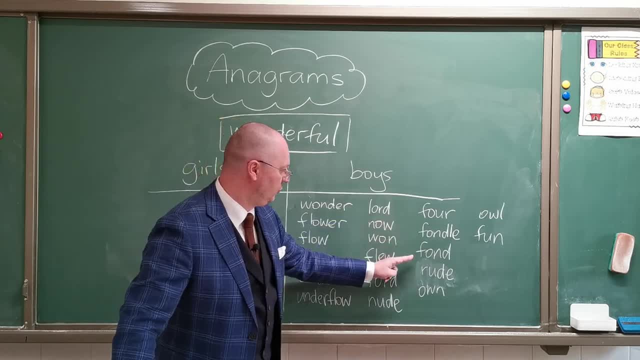 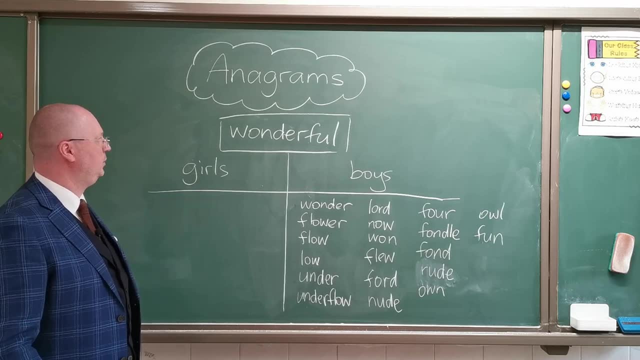 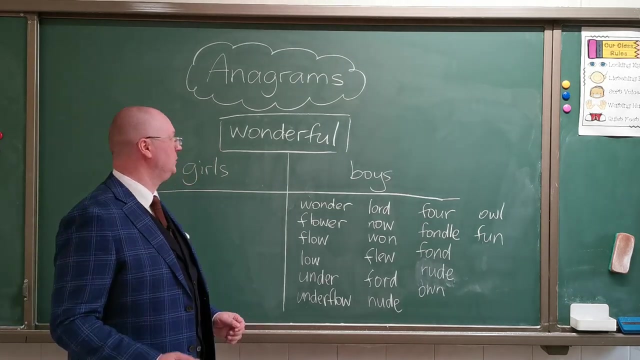 flu fort newt for fondle, fondle, Root own owl and fun. I think there are lots of words that you can come up with here. As a teacher of course I can see maybe more difficult words, but students can come up. 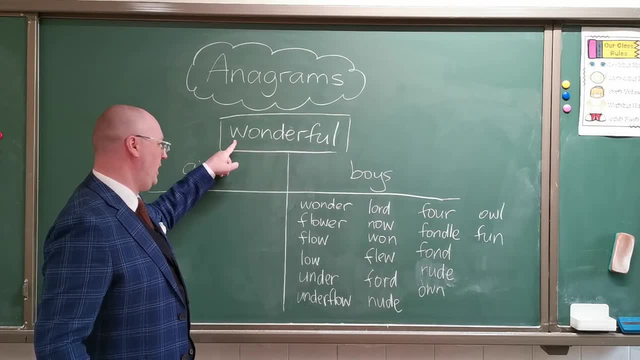 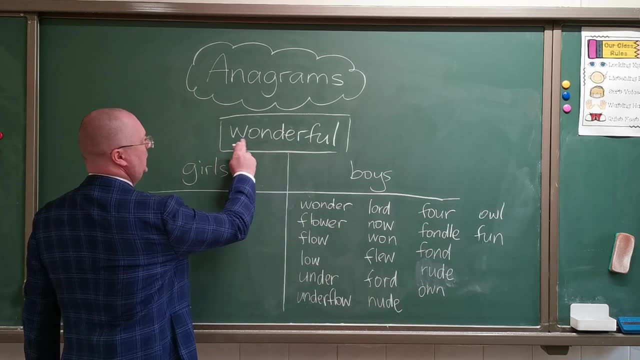 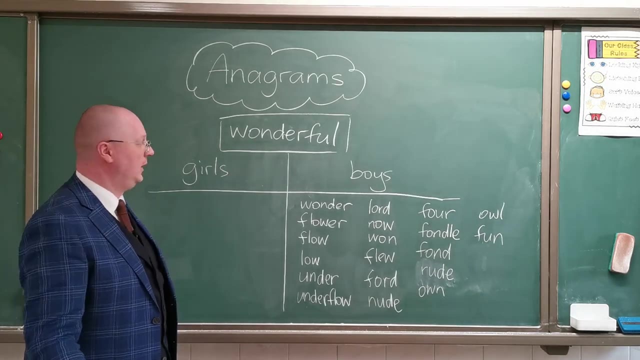 with on or no. now Do I have now I should have had now. That's an easy one. Yeah, for example, N-O-W now And then, if you read it this way, it's One. the past tense of win, right. 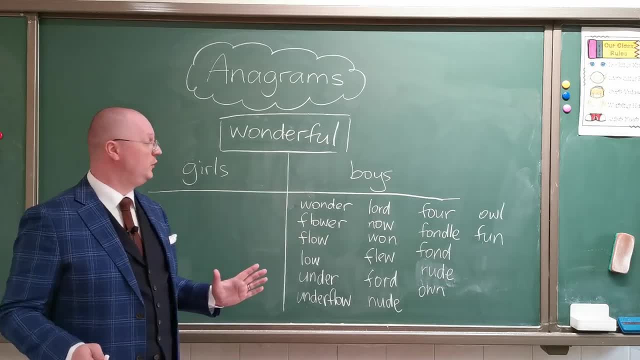 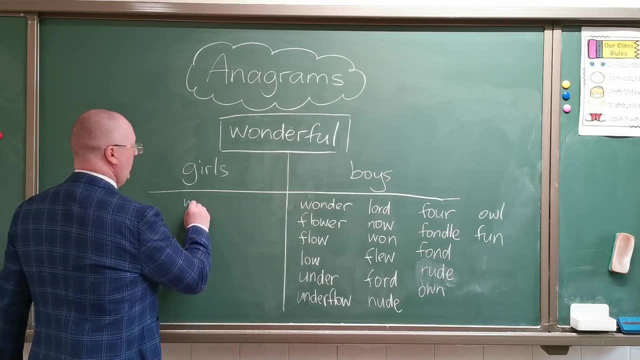 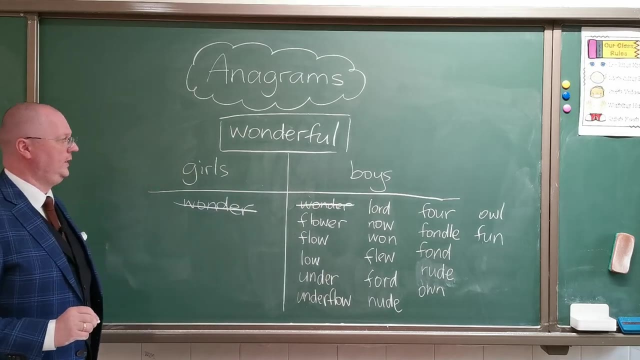 So and then you can like, after you finish this, you can compare. So, for example, if girls have the same word, let's say girls have wonder, yeah, If they have the same words, then you remove this word, you erase it. 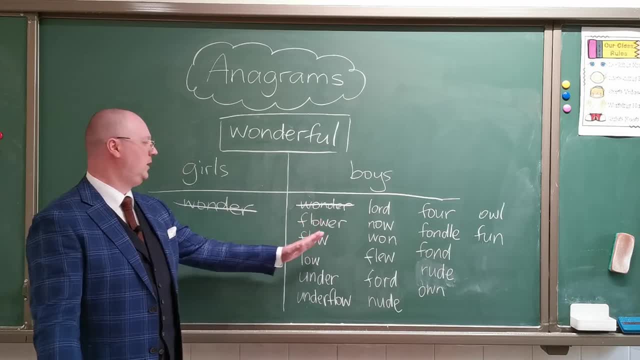 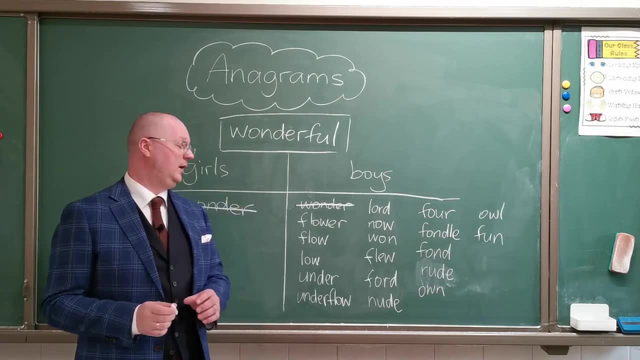 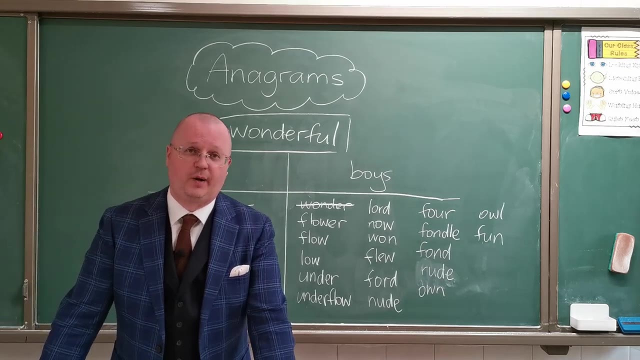 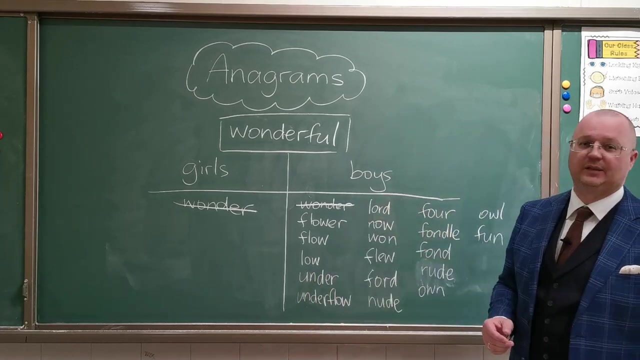 And you only count the words that are not repeated in the team. This is really a great vocabulary building activity because your students can surprise you really. They can come up with really interesting. you know words. They can see it really really well.